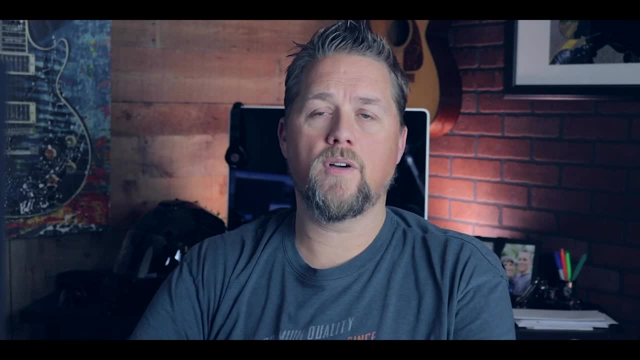 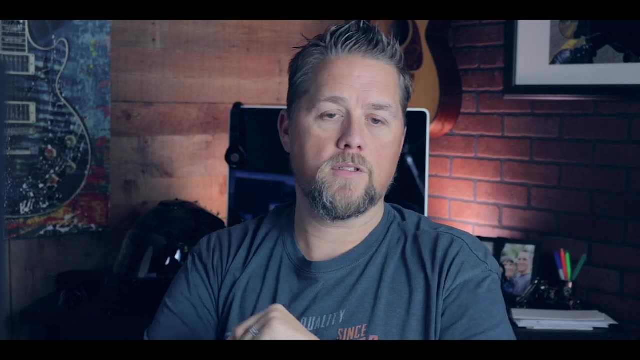 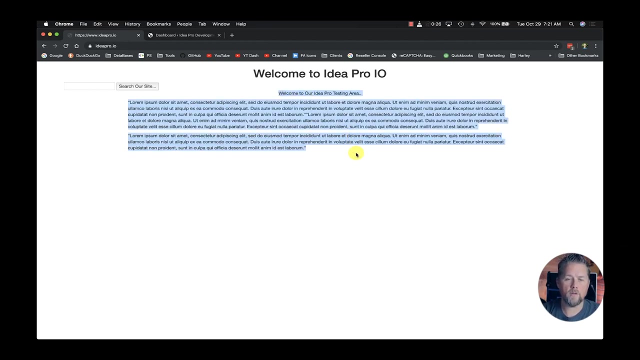 So I'm going to show you guys how to write a quick little function that will minify the content of the HTML from WordPress. All right, so let's get started. So here on our ideaproio site that we do testing and stuff, we have some content here on the front page. 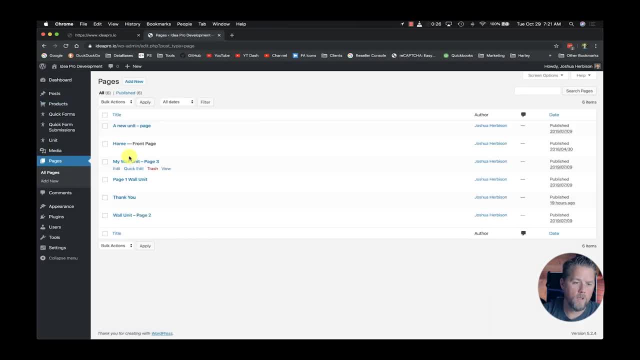 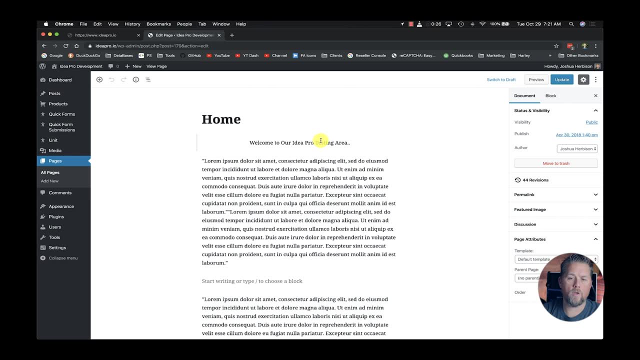 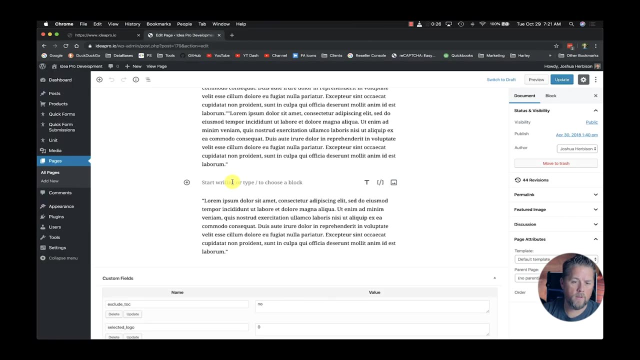 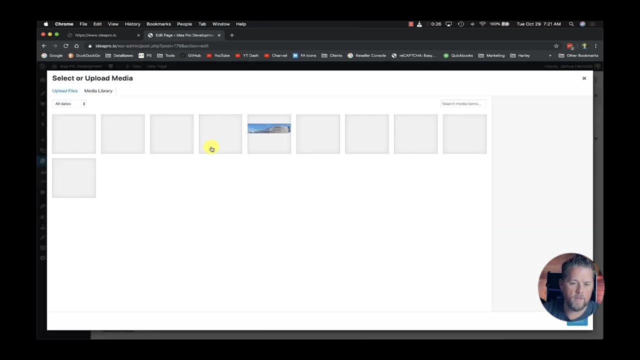 So we're going to go to pages and home page And this is our page here that has a welcome message here and a couple of lorem ipsum paragraphs that show up here, right? So we're going to add: let's do an image, Let's just find something in the media library. I have no idea what's in here. 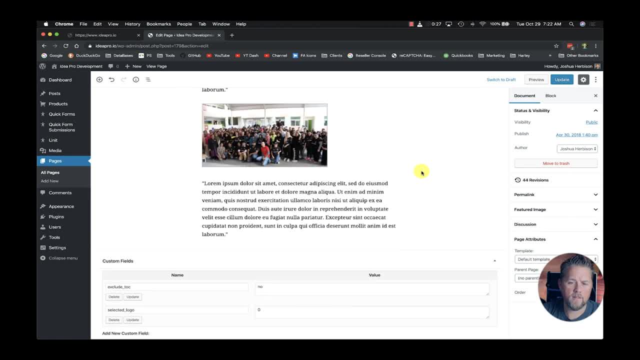 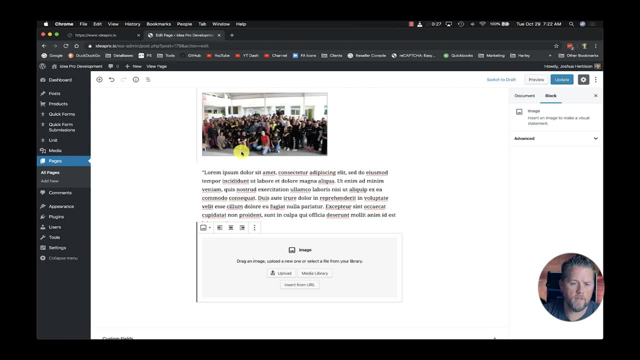 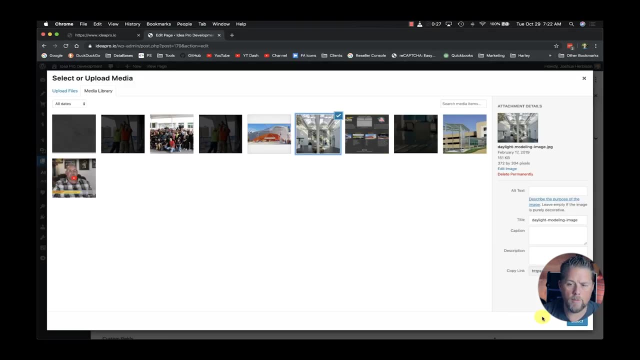 A random picture of somebody, So we're going to put that in there. We're going to come down here and we're going to do a another image. image There it is. And no, I don't want to upload. cancel media library. We're just going to add this image in there, All right? 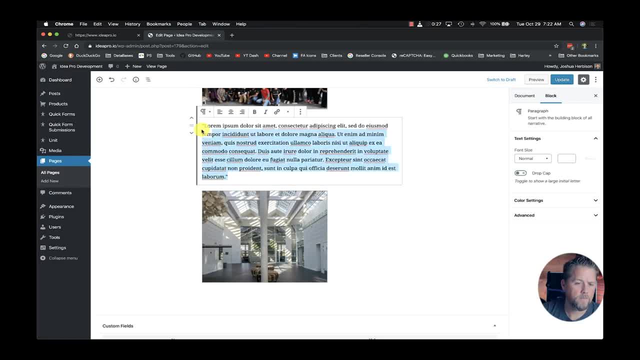 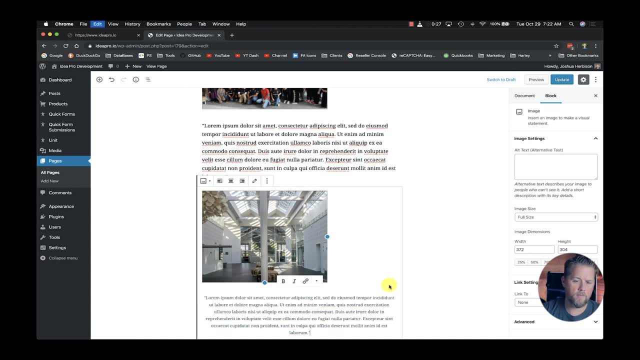 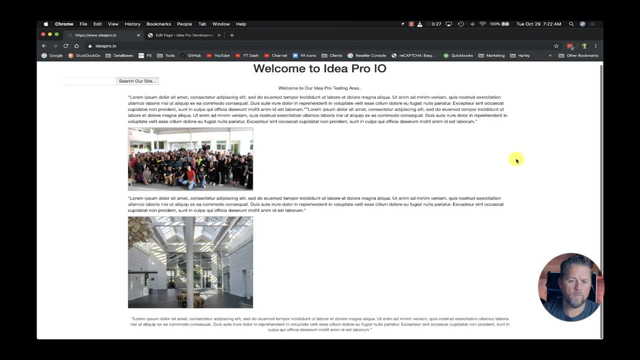 And so then if we copy this text here, this lorem ipsum here, and come down here and paste this text, All right, So now we've got some content on this page, Let's go back here and refresh, All right, So now we've got some content on this page. Definitely not optimized. 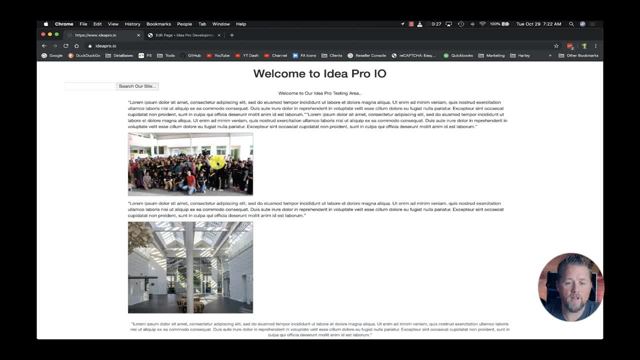 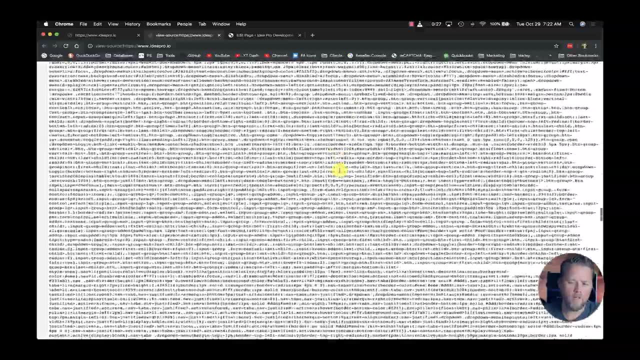 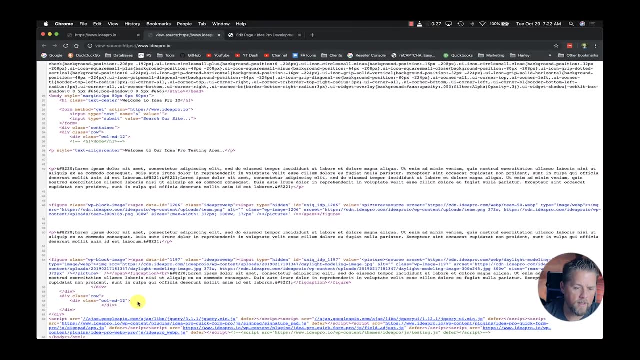 Those images are really really large. Um, they're not showing up very large, but they're they're pretty large. And if we view the page source, come down here, a lot of our sites are optimized already by plugins and stuff that we've built as we come down here. Now we've got um. 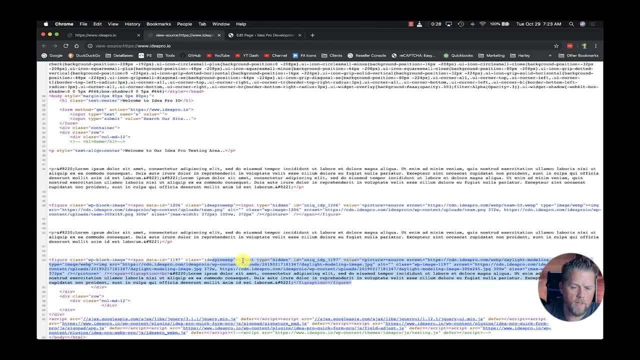 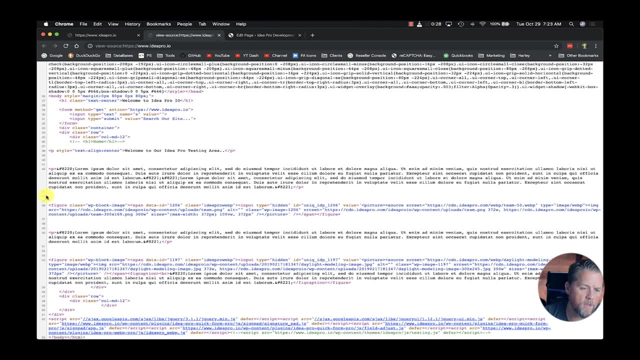 this here, which is the lorem ipsum uh and an image tag and a paragraph tag, And so there's a lot of white space in here. We've got one, two, three, three blank lines in between each one of these uh paragraph tags, or this figure tag and the paragraph tag here. 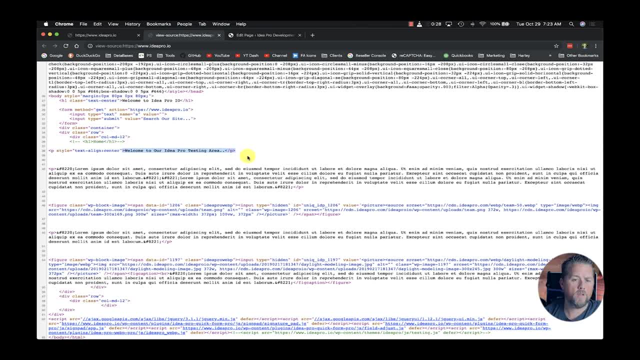 So we've got a lot of space in between. you know, welcome, the welcome message. Then we've got three lines of blank text, which is insane that it puts that many um blank lines in there, But it does All right. So I'm gonna show you how to write a quick. 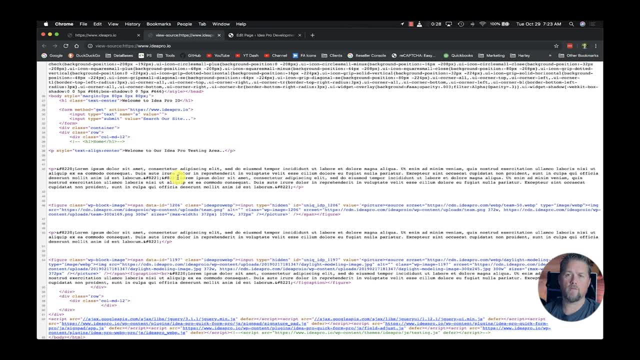 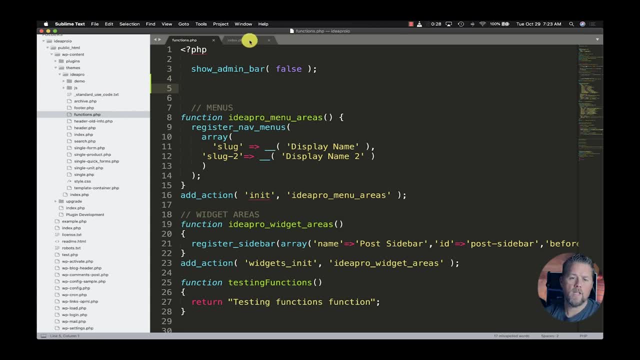 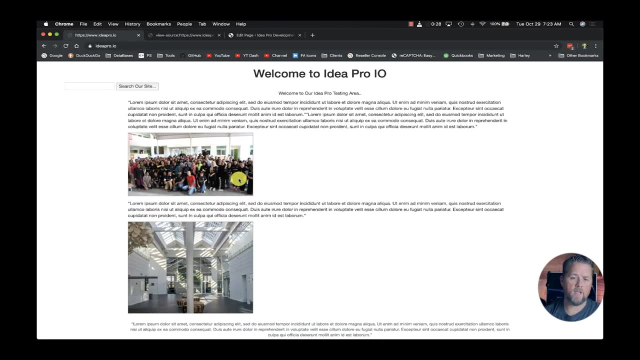 function that will optimize the content coming from WordPress. All right, So let's go to our development area and we're in our functions- dot PHP page And then we have our index dot PHP page here, which is the default uh page, which is what's running this page here. It's the 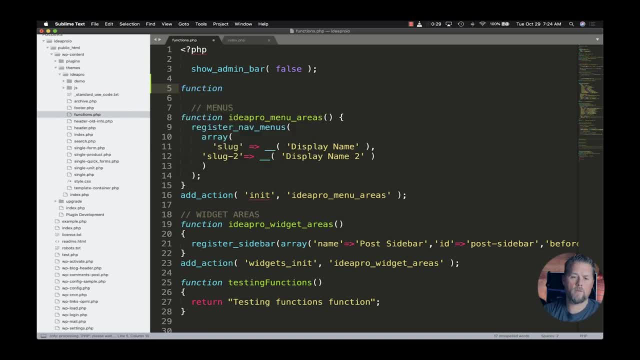 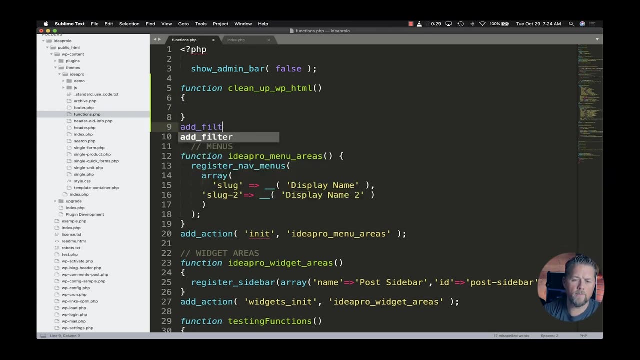 go to our functionsphp page and we're going to just write a function, so we're going to say: clean up, wordpress, wp, html can be any name that you want to name your function there, all right. and so then we're going to add a filter, oops, and then tell it what we want to filter and that what we want to filter is the content. 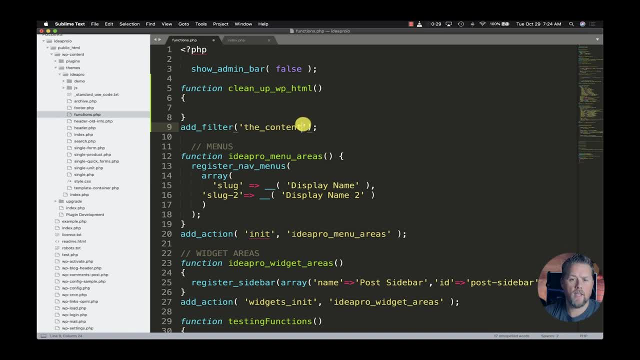 okay, so add, filter the content, and then we're going to do our callback function here. so when we filter the content we want to run this function. now the attribute inside of our function here needs to be a variable, and we're just going to call it content, so that in here we can now 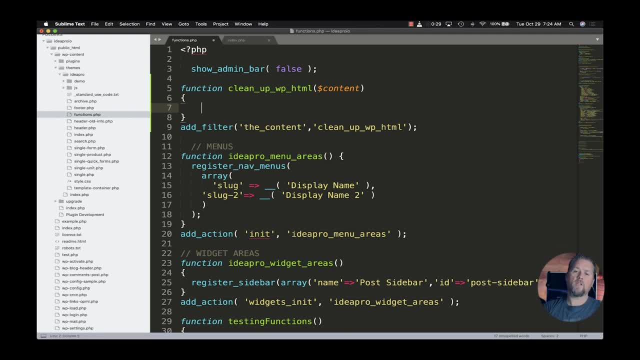 make manage that content, we can add to it. if we want to add something to every page in our entire wordpress website, we could say: content is equal to dollar sign content. oops dot, and we'll add a break. thank you for visiting our page, right? if you didn't build your theme and you want to add something to every page, you can do some. 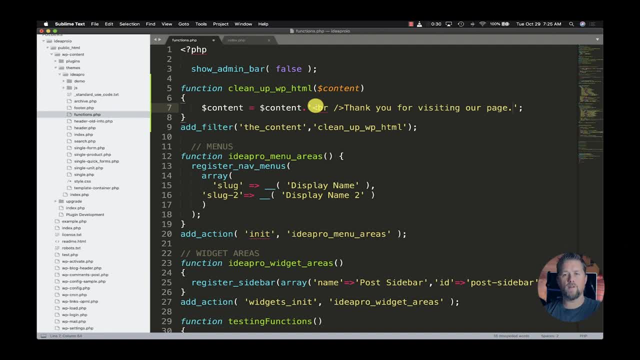 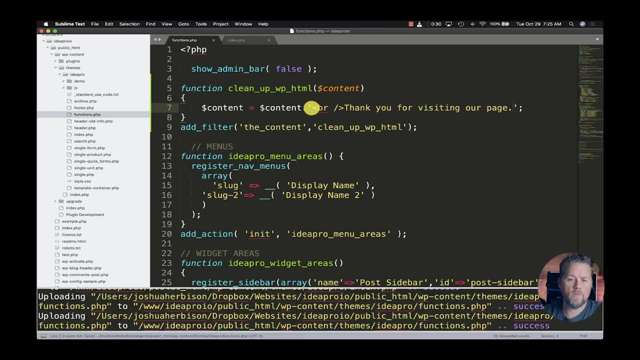 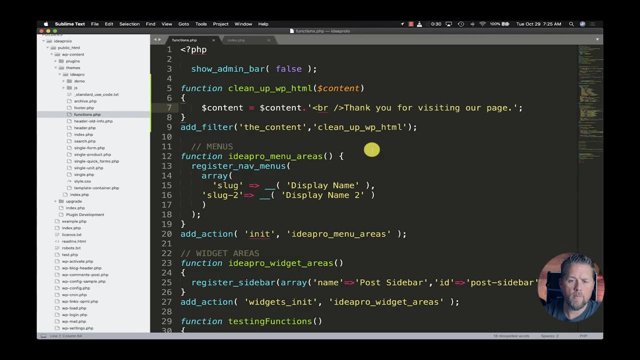 something like that. if you don't want to edit the footer- you know the header, the footer or each individual template- you could just add a filter to the content, right? so if we save this, come back and go back here and we refresh and we got a problem. 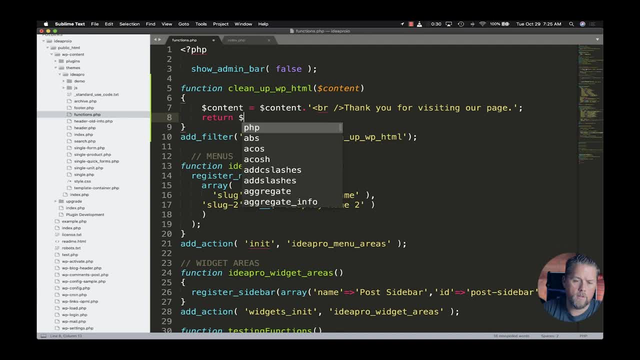 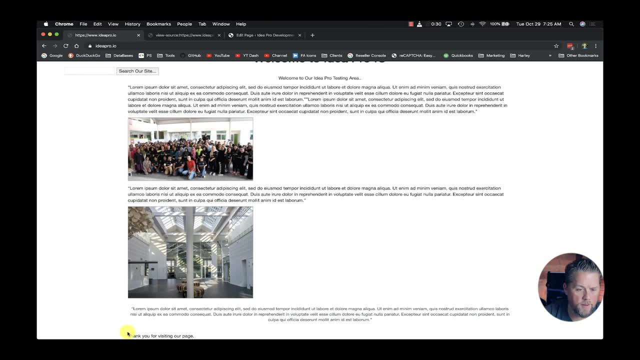 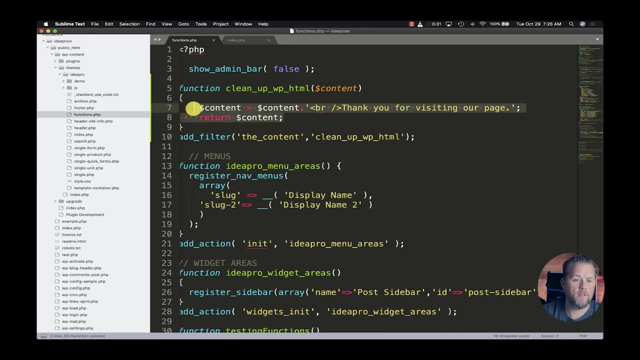 oh, didn't return the content. return content. there we go. so now we have the regular content and then down here at the bottom, thank you for visiting our page. all right, but that's not what we're talking about here. what we're talking about here is we want to edit the content to clean up. 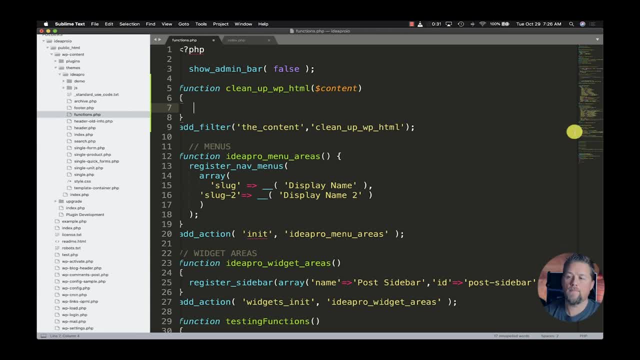 and remove any of the white space. all right, so this takes a preg replace and i have a copy of it over here because this is something that you really it's hard to keep up with- of what each individual- and i can do a video on preg replace of each individual code that goes. you know what? 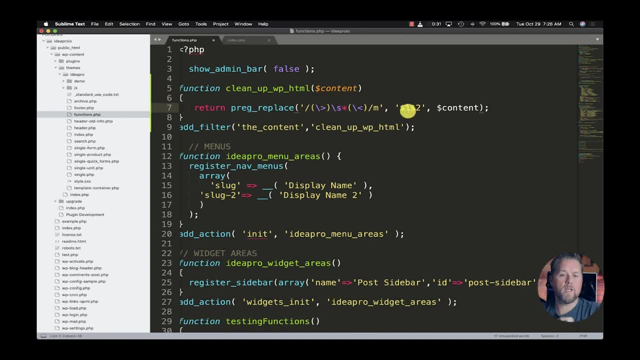 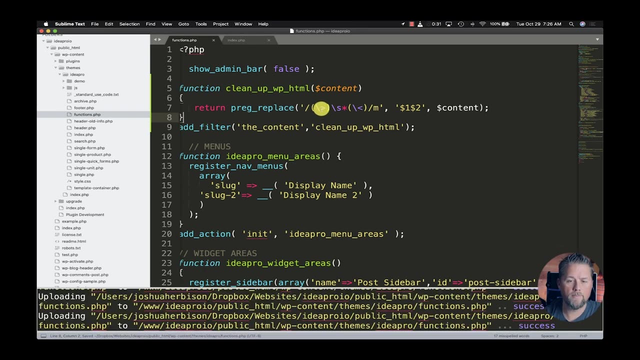 each individual little uh character does. but so basically preg, replace, and then this little bit here, dollar sign i, dollar sign two, and then the content, and we're returning it here. so that's really the only line of code that we need. all right, so we come back here, we refresh, we see that. 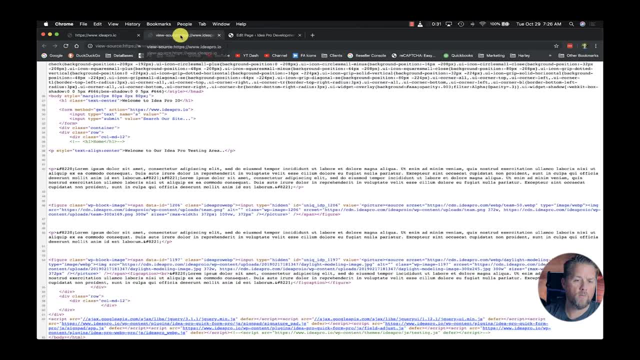 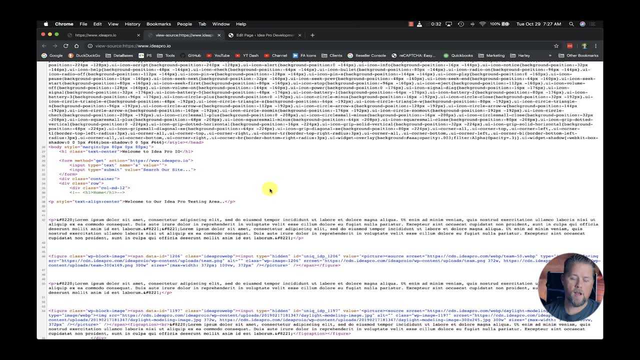 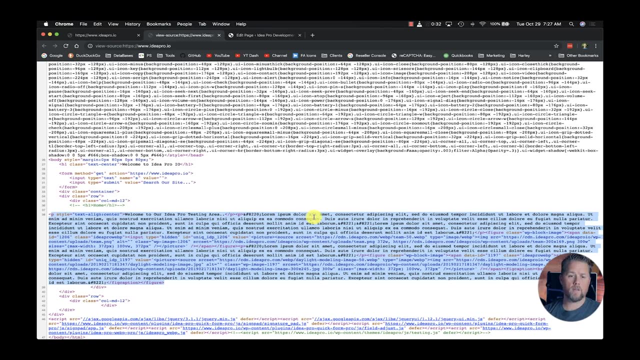 our page is still loading normally and we go back over here. if we look, we're at 63 lines of code before the optimization, and now we hit refresh. and so now you see, all this html is optimized, it's all minified, and now we're at. 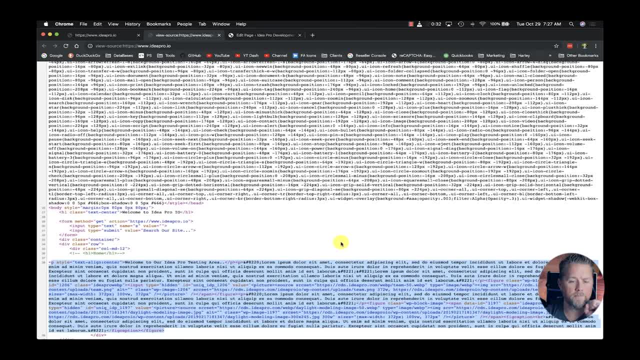 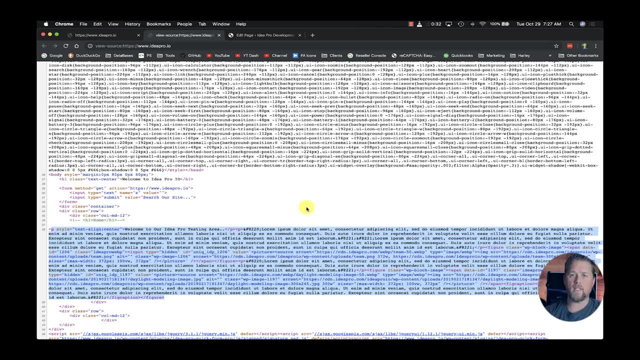 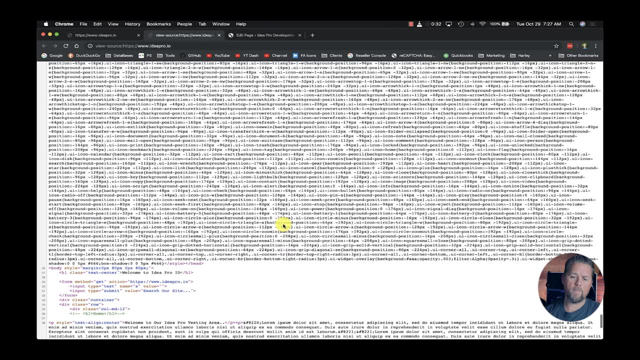 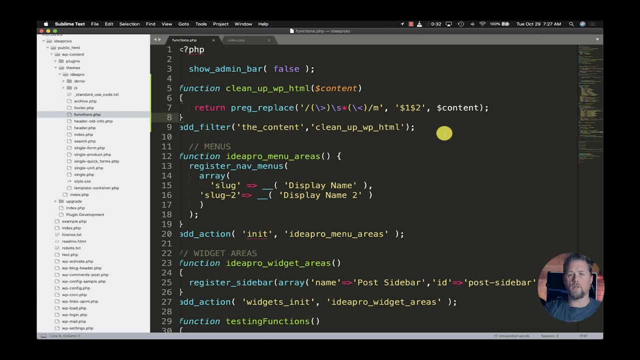 a total of 47 lines of code. right, so we've basically taken out almost 20 lines of code or 20 blank lines from the the code to minify the html for our wordpress. all, right, now you can build this into a plug-in, which, what we do, we build into a plug-in that we use on all the sites i will. 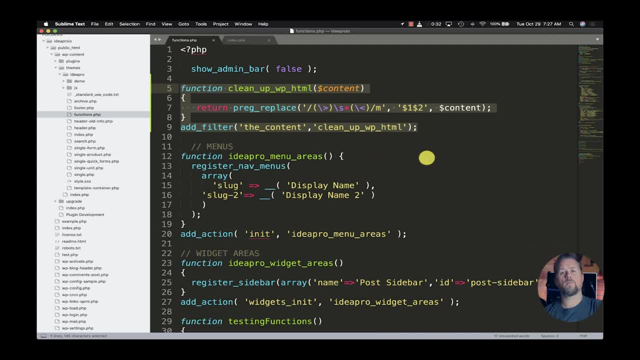 include this code in the description down below and if you need to know how to build a plug-in, i'll link the card up here and the video in the description on how to build a plug-in, and you can include this function on any of the plugins or you can include it on your functionsphp. 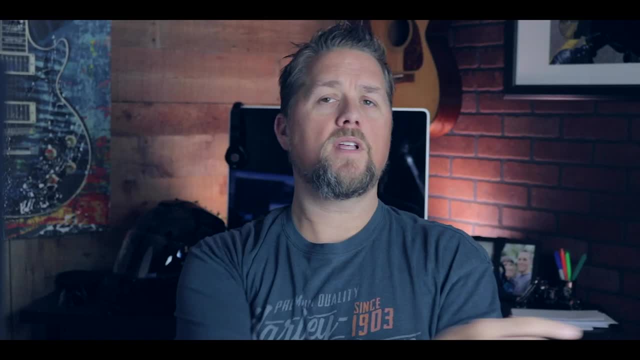 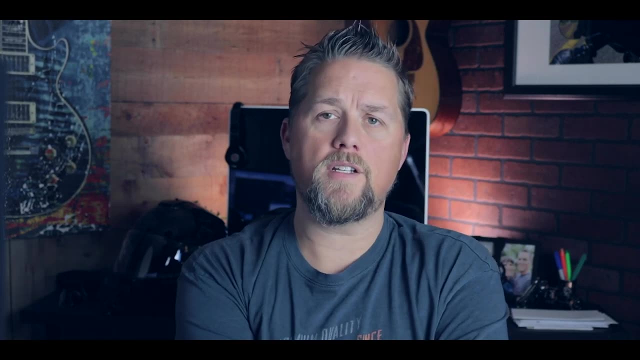 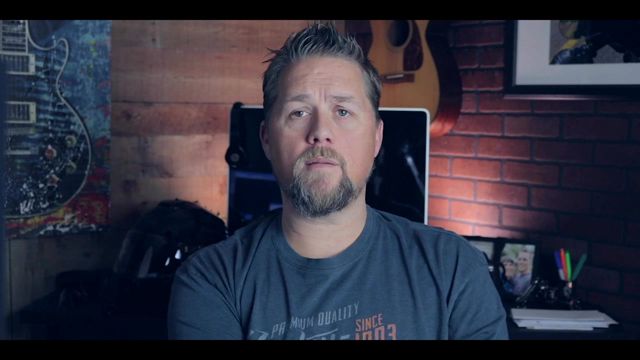 file and you're going to be good to go, so hope you like this video. share it with anyone that you think will learn from it or will benefit from using that to minify their html in their wordpress website, and click the bell for notifications- subscribe. leave me a comment for videos that you want me to do, and i'll see you in the next video.